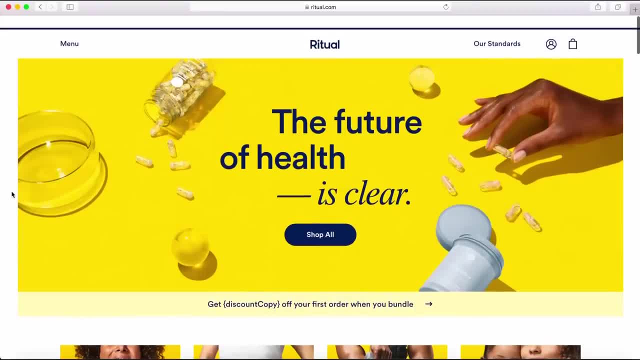 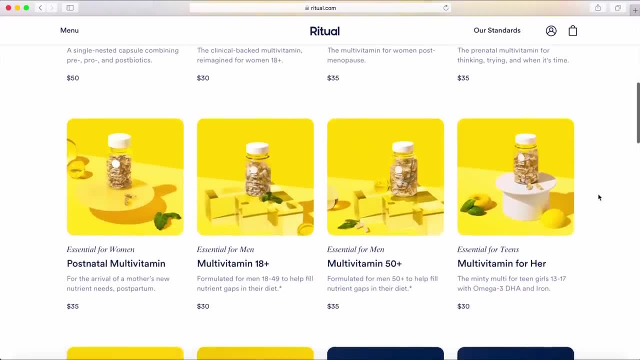 basis. That's where Ritual has filled this gap for me. Were you ever skeptical in the past about needing a multivitamin, or did you always assume a healthy diet was enough For me? I always did, until I did further research. Ritual has developed their multivitamins as they offer a delayed release. 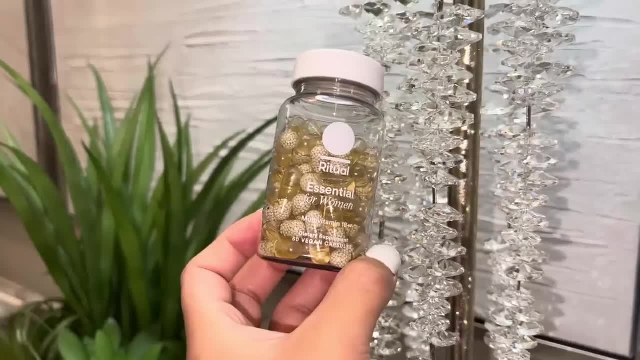 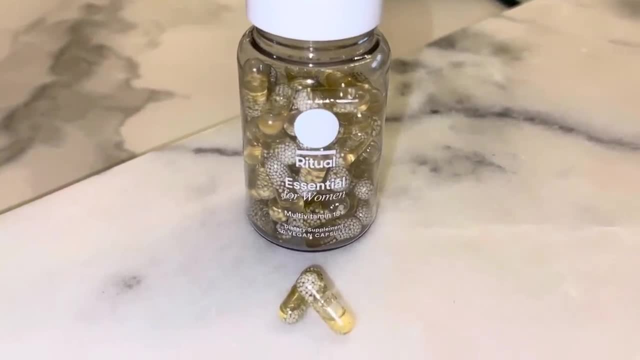 capsule design. This means the capsule was designed to dissolve later, to help bypass the stomach and dissolve in the small intestine, making it an ideal place for absorption. This is Ritual's essential for women. 18 plus multivitamin: Many of the vitamins important. 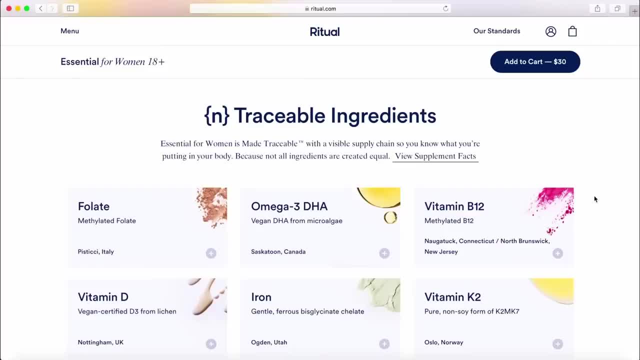 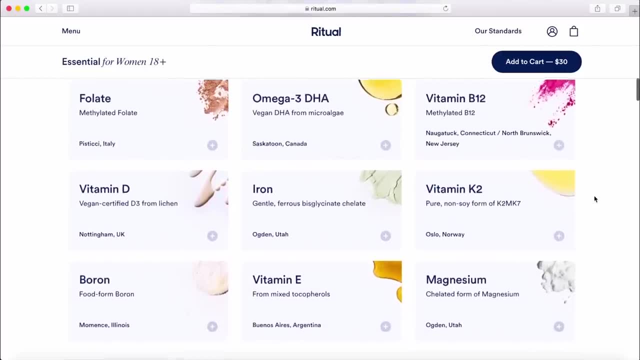 to me in this capsule is the omega-3 for brain health and vitamin E for fighting antioxidant support and fighting free radicals. I love that Ritual uses clean ingredients and they're transparent about everything that goes into the vitamin. that's why they're clear. Taking a multivitamin is like a nutrient backup plan In the areas 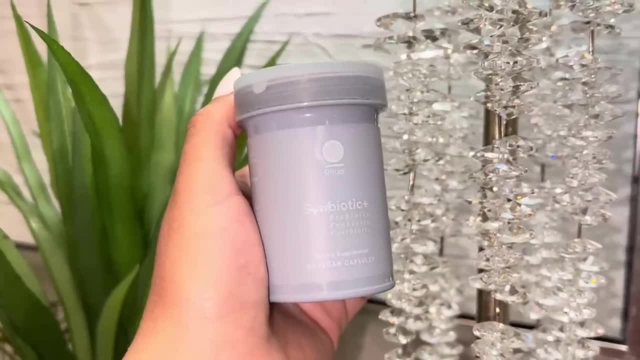 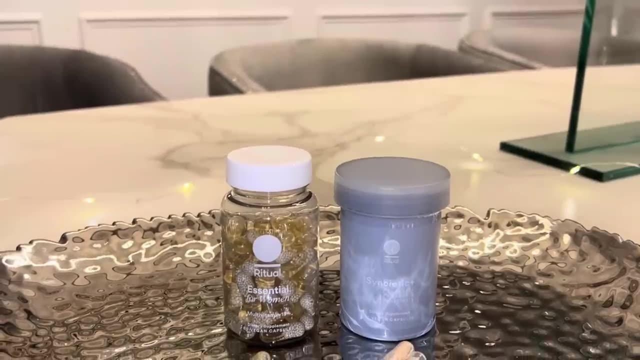 where food falls short. getting support from a quality multivitamin can help fill nutrient gaps, no matter the dietary preferences, age or current life stages. These vitamins are vegan-friendly, gluten-free, formulated without major allergens and non-GMO. Make sure to. 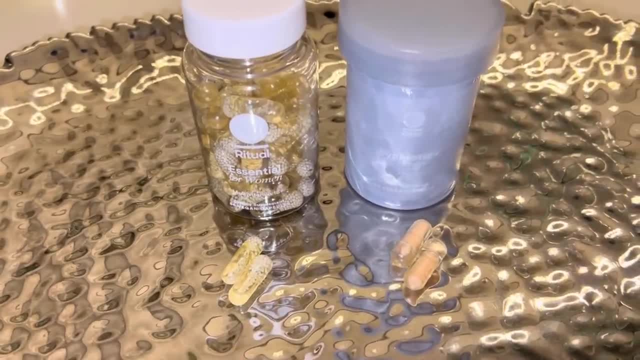 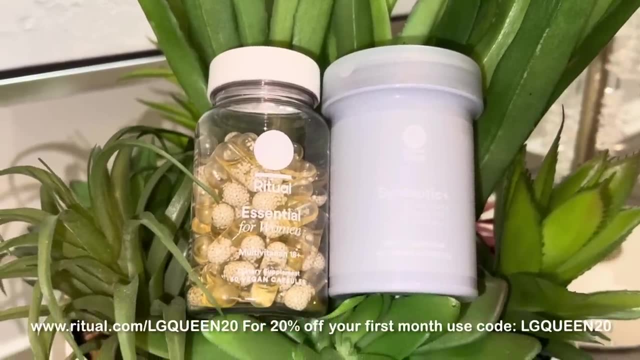 check out my description box, where I'll leave a direct link to shop this incredible multivitamin and more. Ritual is giving my viewers a special offer of 20% off your first month. All you have to do is enter the code LGQUEEN20 at checkout to take advantage of this special offer. Thank, 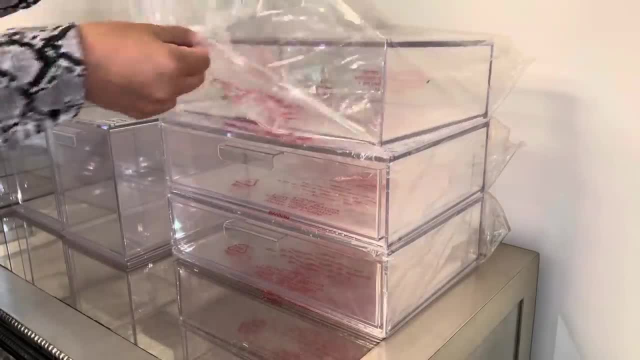 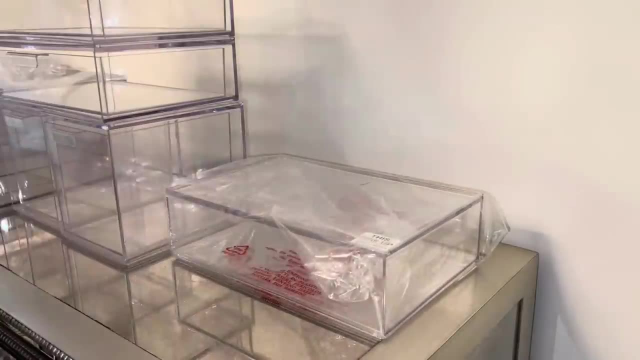 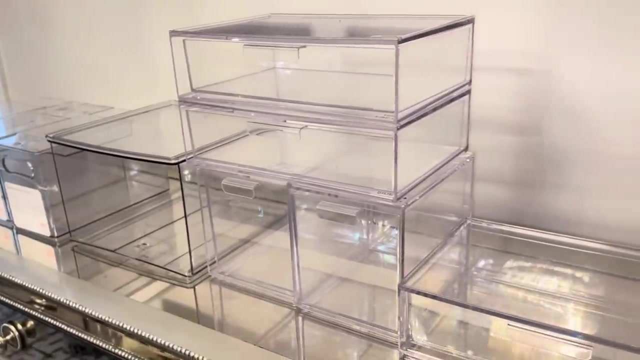 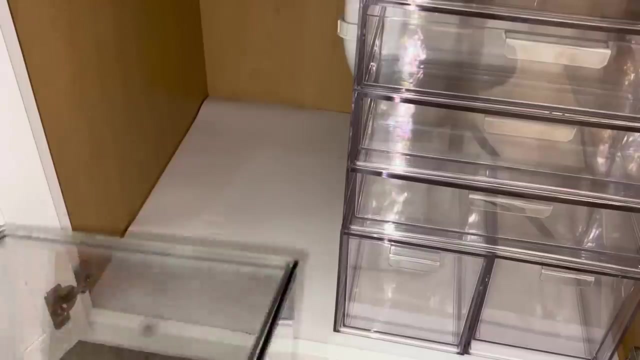 you to Ritual for sponsoring a portion of today's video. now let me show you guys how I transform my bathroom with the ultimate organization. I'm going to take a few seconds to show you guys that look how beautiful my bathroom is using the Thermogen había. 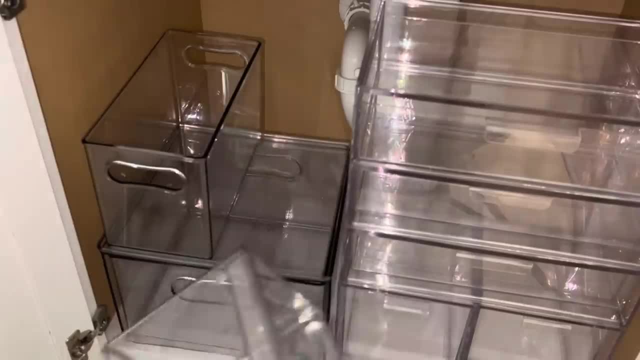 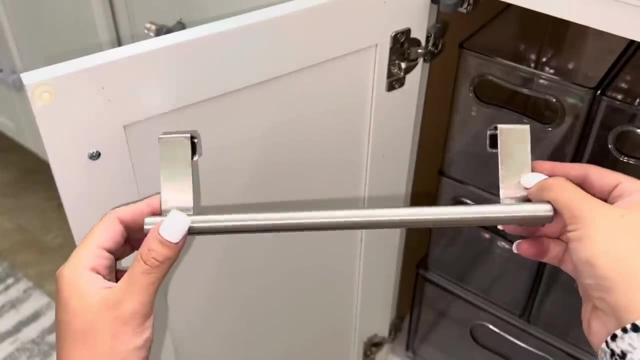 It's very simple and you get a good natural color bath. I hope you have a lovely and healthy evening. Maybe you'll actually get a better night's sleep if you do that. Thanks again for watching and we'll see you next time. Have a great day. 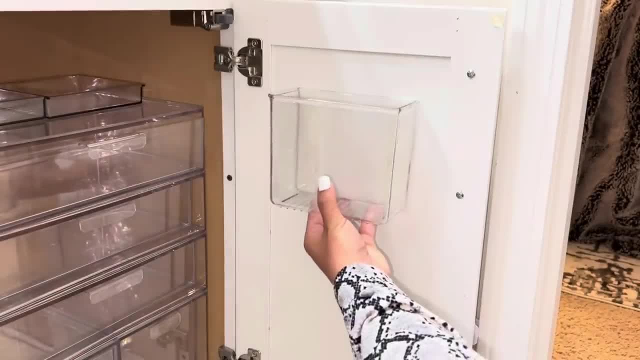 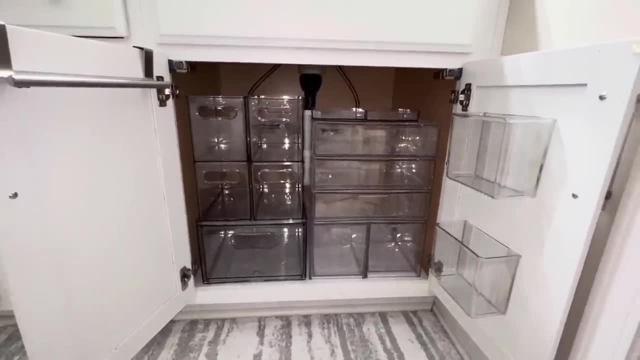 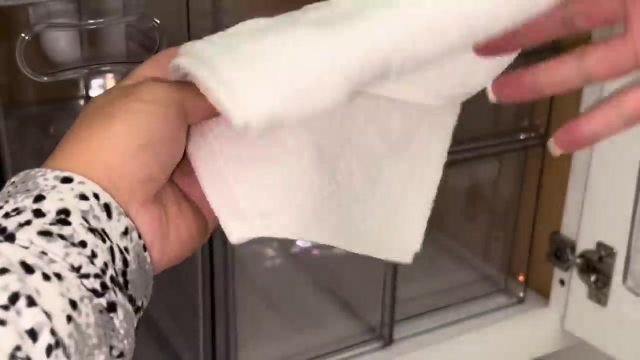 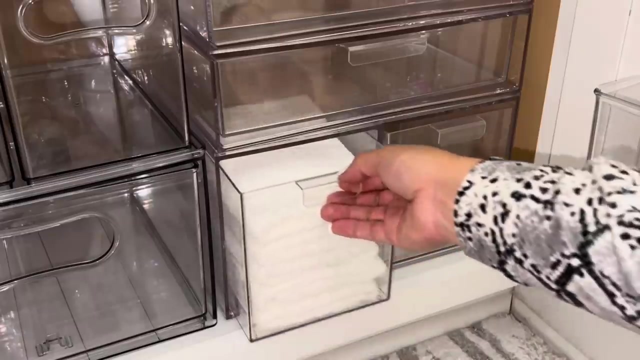 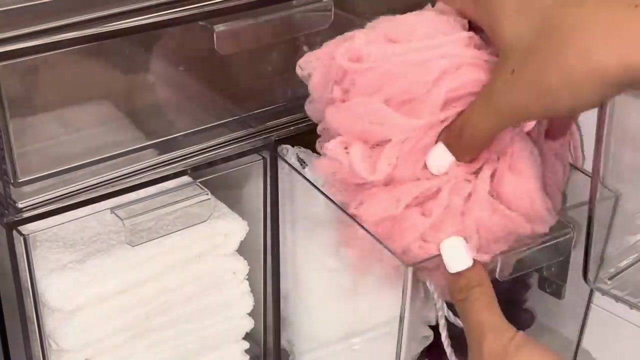 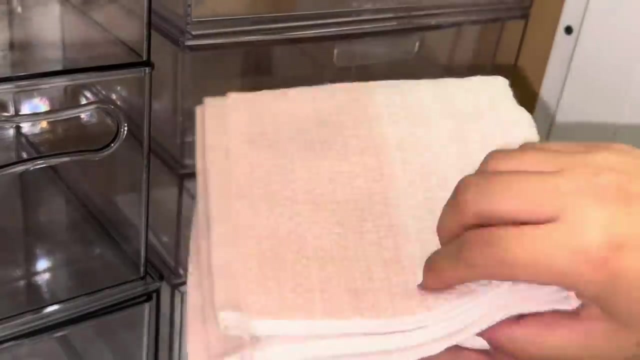 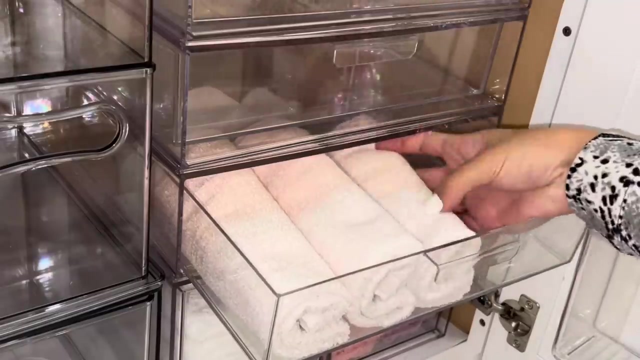 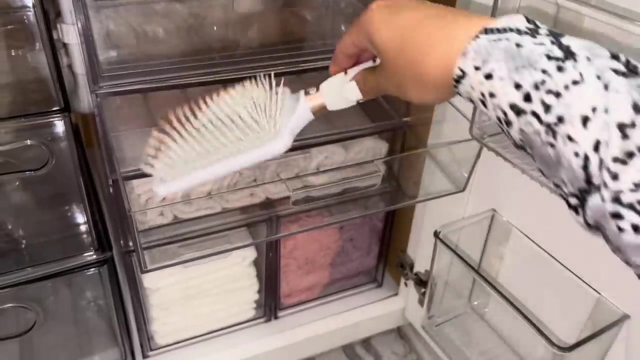 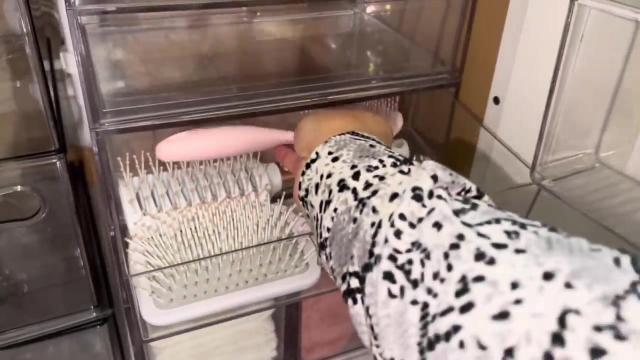 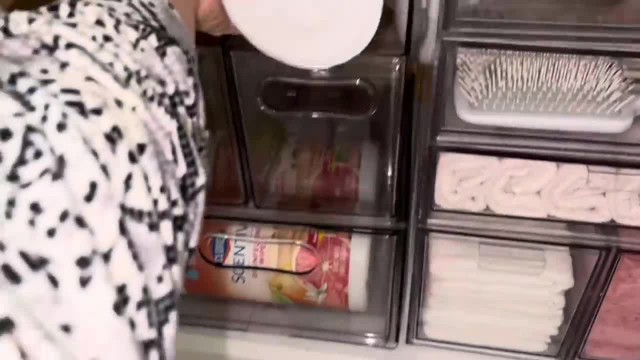 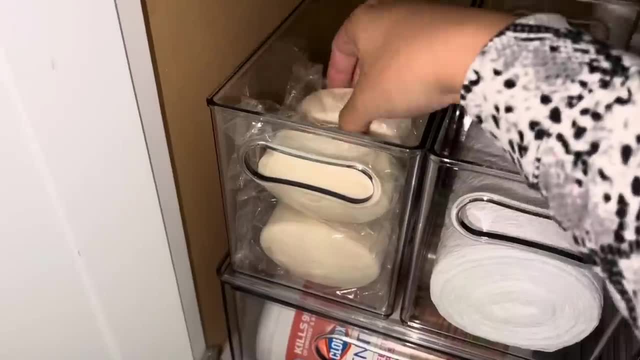 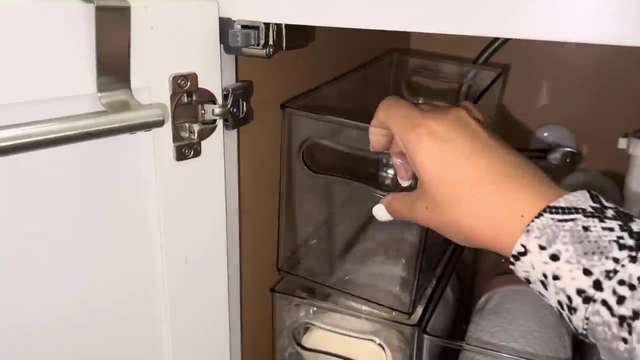 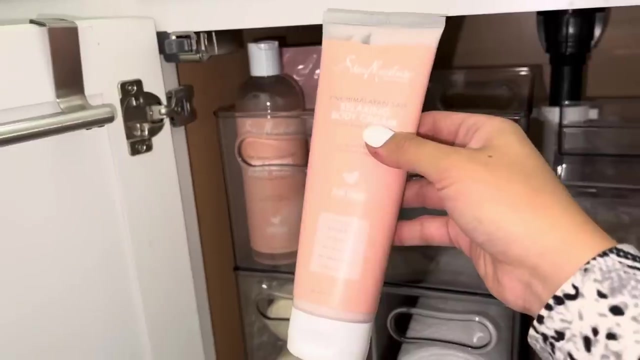 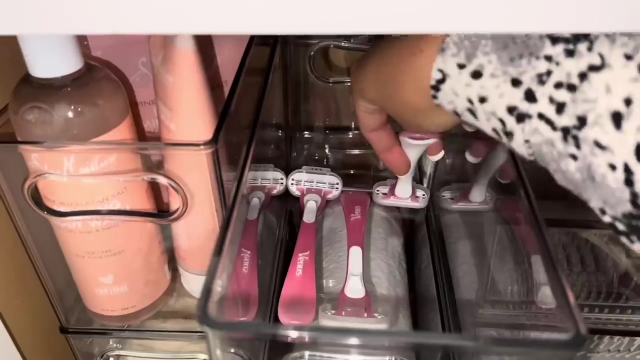 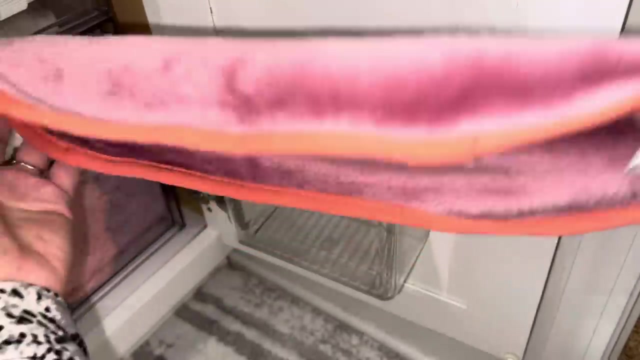 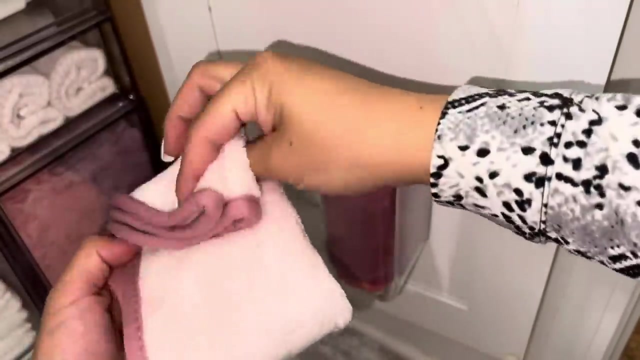 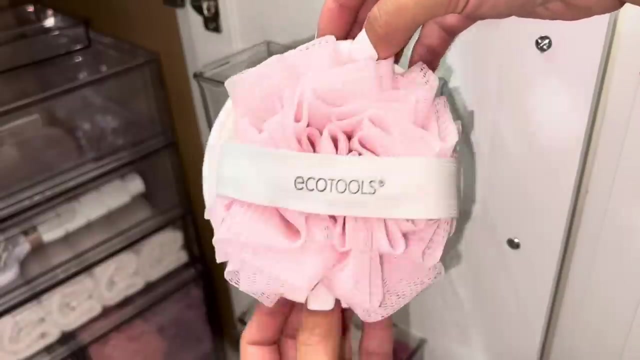 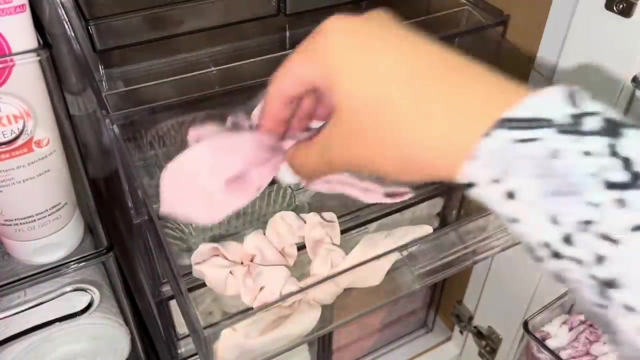 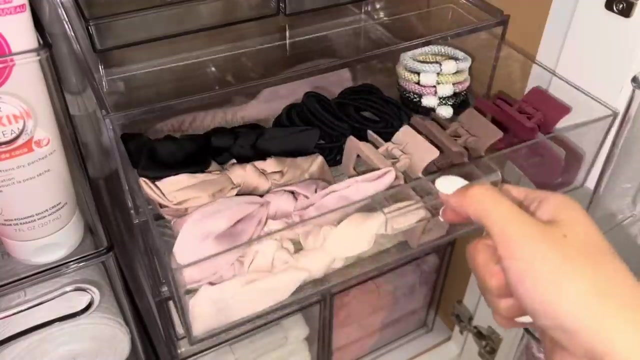 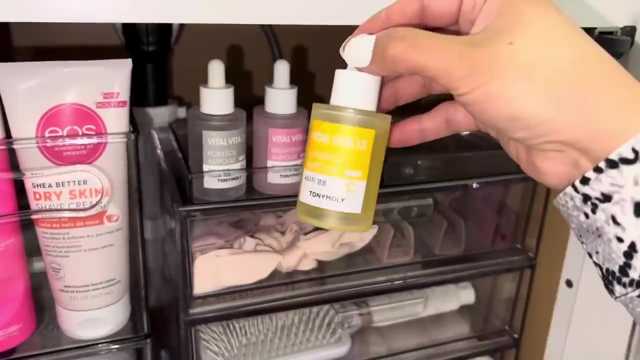 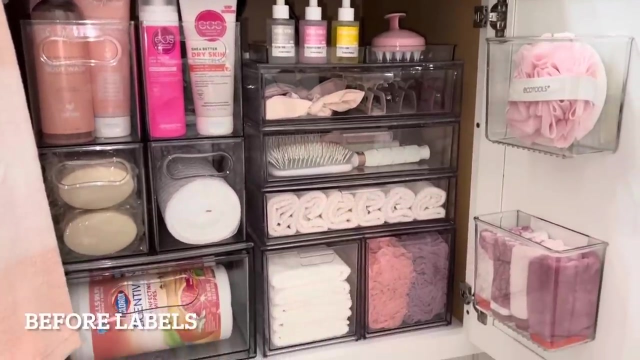 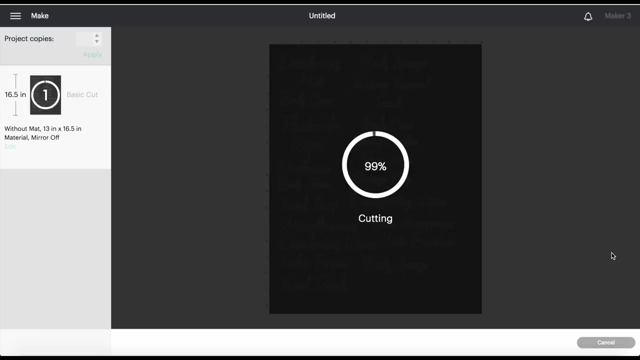 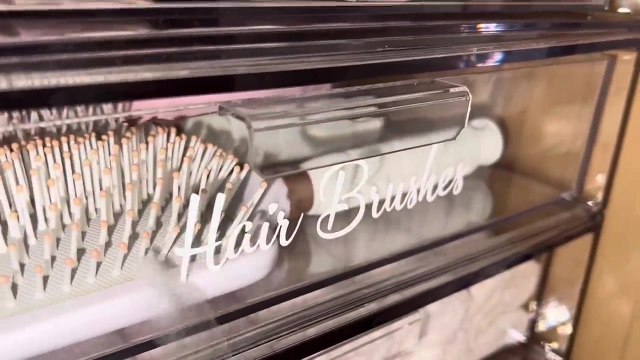 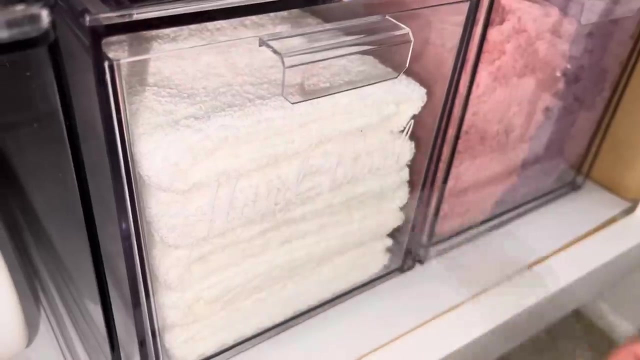 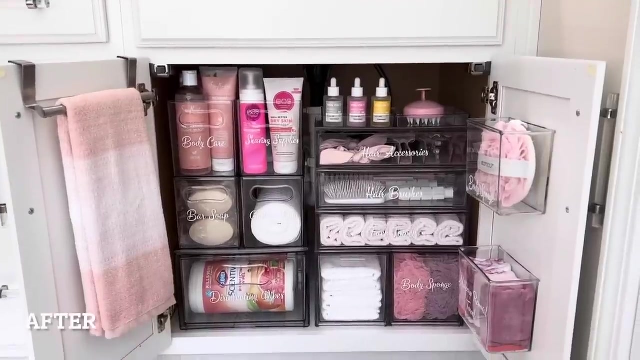 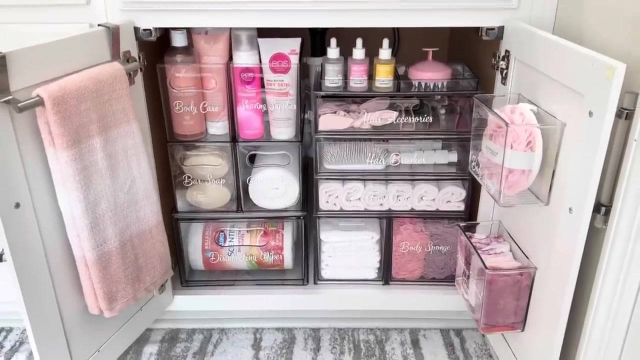 Thank you, Thank you, Thank you. Here's a look at the before and here's the after. The end result is always so satisfying to see. I love the way the space turned out. I wanted to maximize this cabinet to fit all of the essentials that were too big to fit in the smaller drawers. 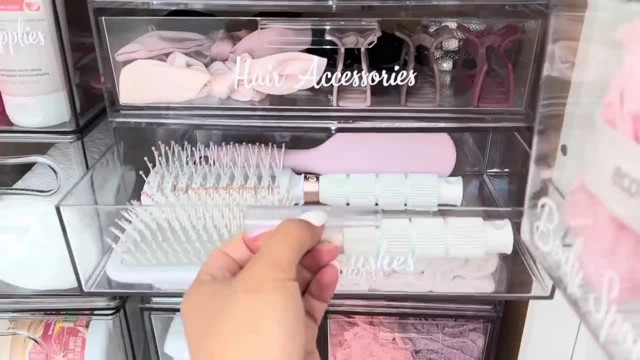 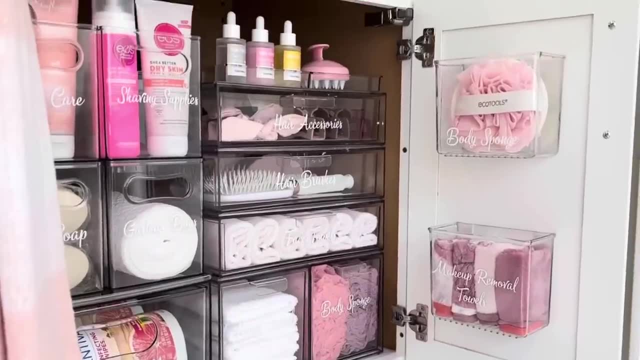 I can now reach anything easily and I can see everything in the container. If you're interested in any of these products and organizing containers, I'll have it all linked down in the description box. Let me know in the comments how you think this space turned out and what color scheme would you go with in your cabinets. 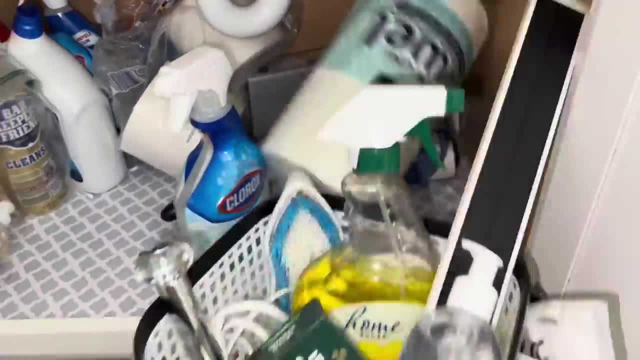 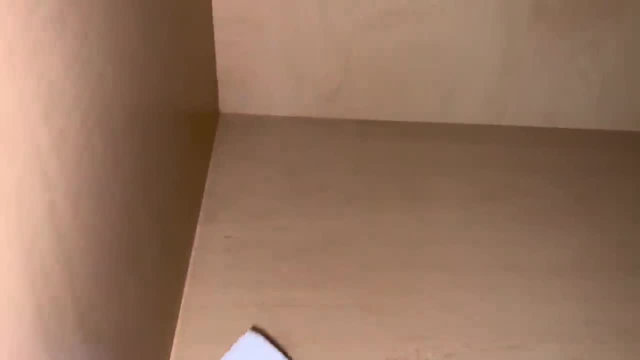 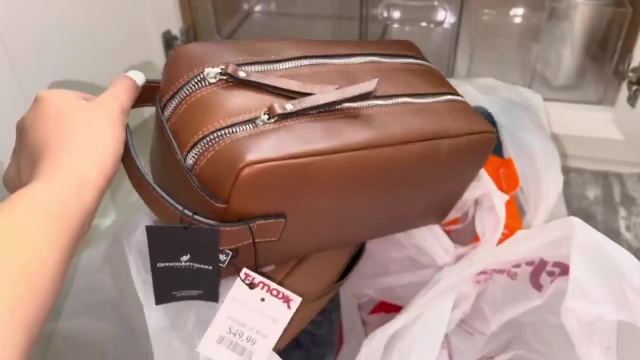 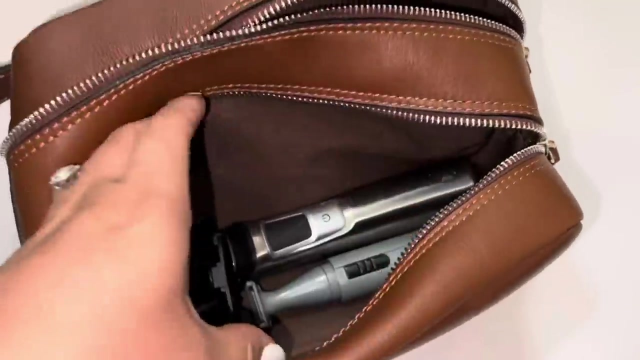 My girl's bedroom makeover in my recent video inspired me to add blush color details in my cabinet. If you have any questions, feel free to ask them in the comments section below and I'll be happy to answer any questions you may have in the comments section below. 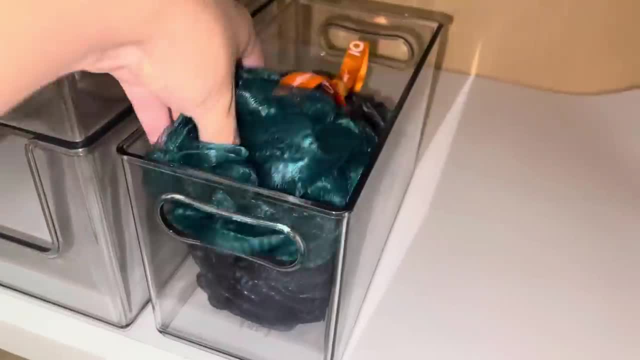 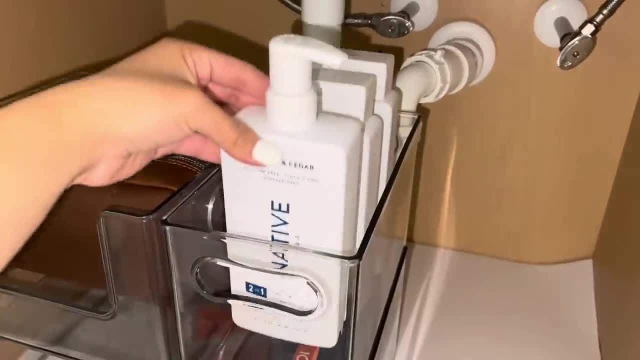 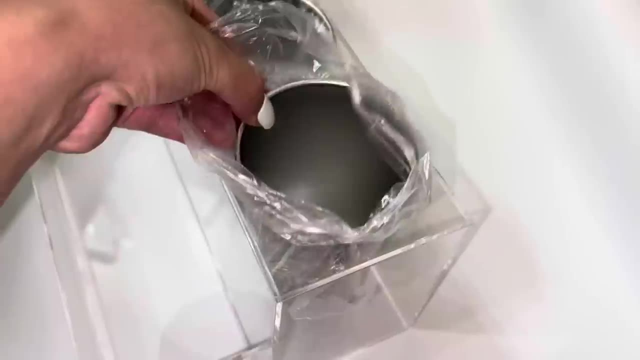 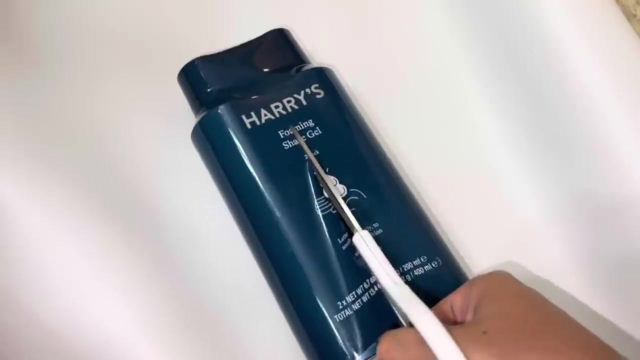 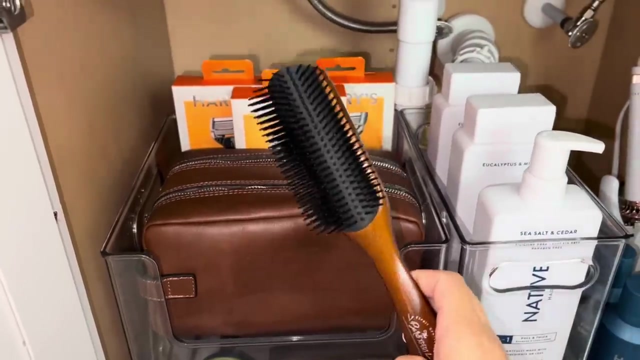 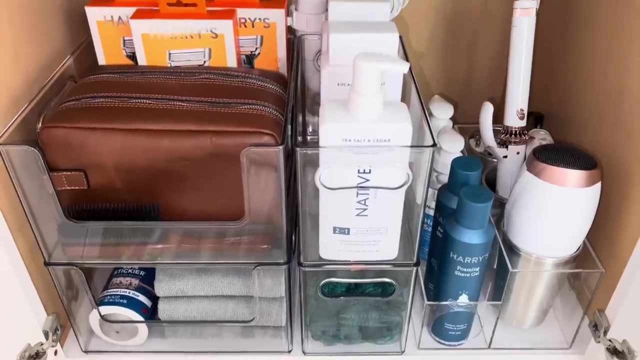 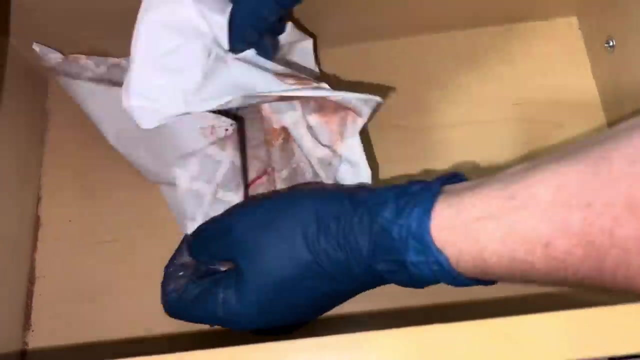 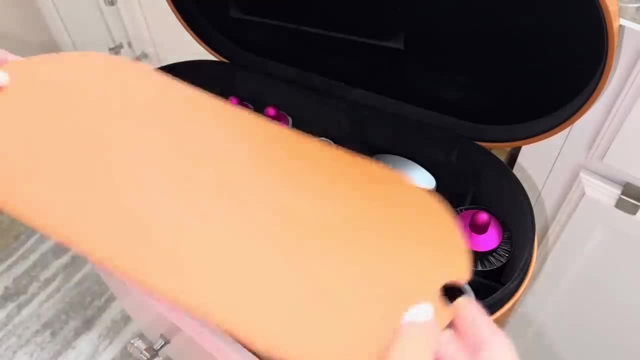 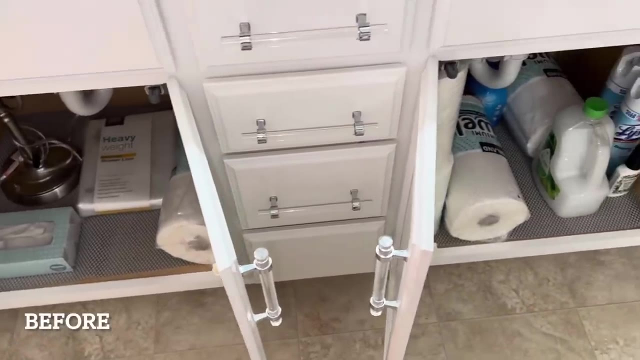 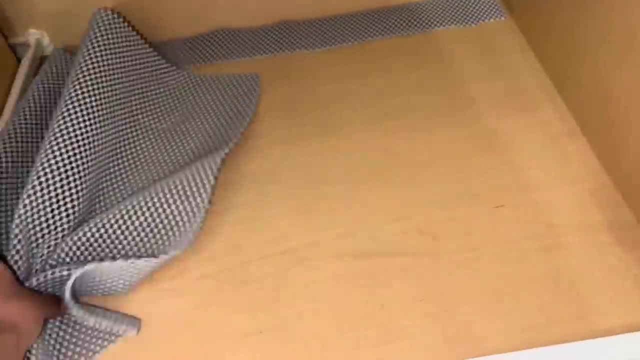 Moving on to the guest bathroom. I had to make a change in this space because it was bothering me seeing things all over the cabinets and drawers. I want my guests to feel welcomed and loved, and this space needed a lot of attention. I started off by removing everything and getting rid of things. I no longer needed to make room for necessary things in this space. 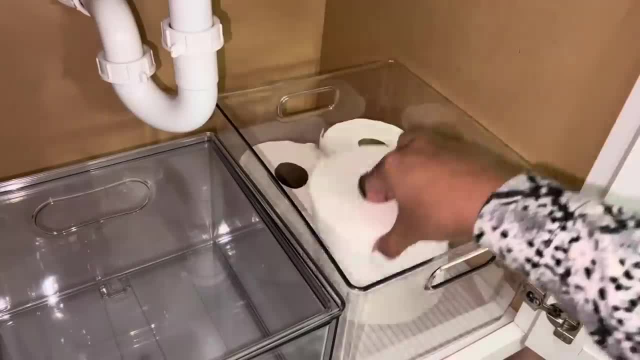 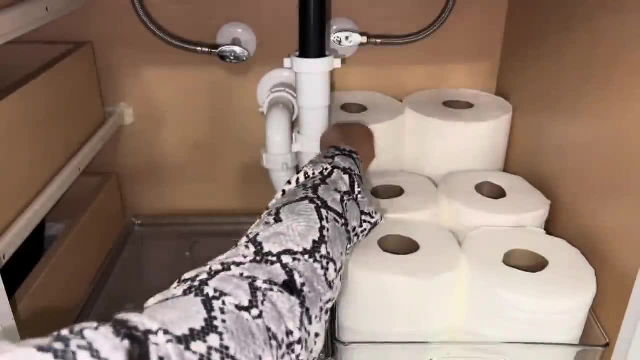 It was a pleasant change of mood, but I couldn't get enough of it. As for my other's room, I didn't have a space to care about, so I planned to convert it into a small room like this. I made a separate room for them, which is pretty much it, but I wanted to give them a sense of community. 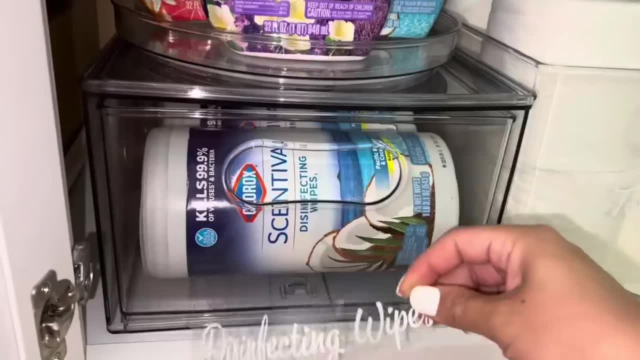 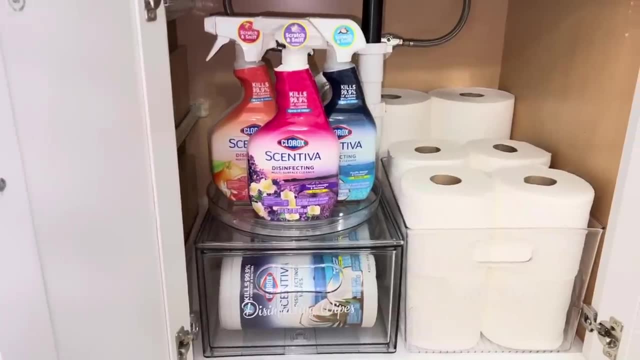 It was very upscale, the ground floor where I built the kitchen and the living room. I decided to make this a little smaller and favored the entire room with a little bit of space. I ended up with a little space for my kitchen and the living room. 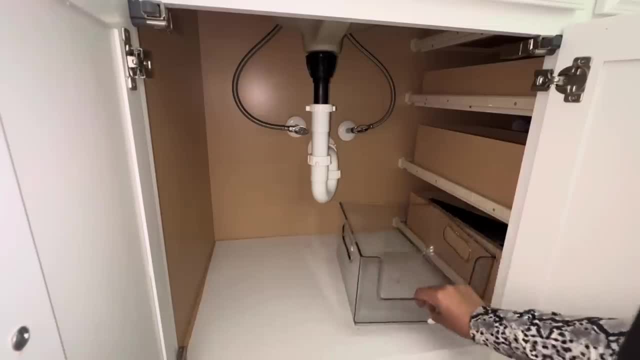 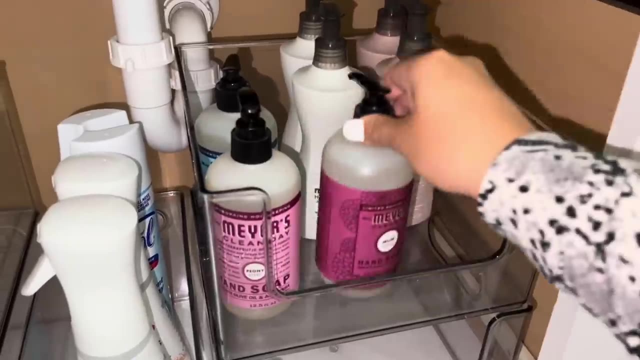 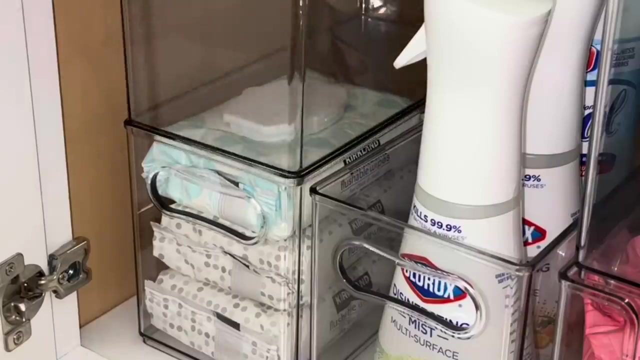 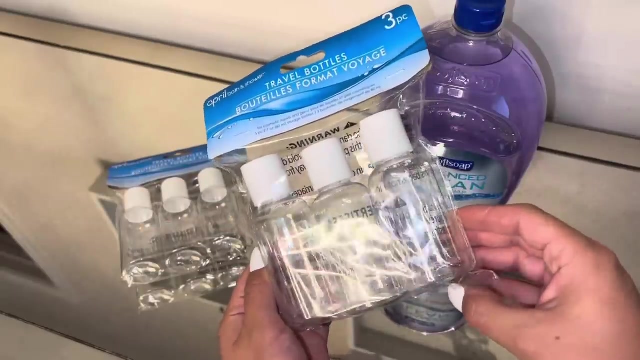 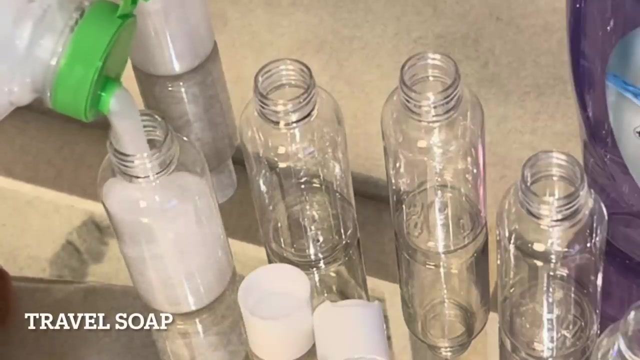 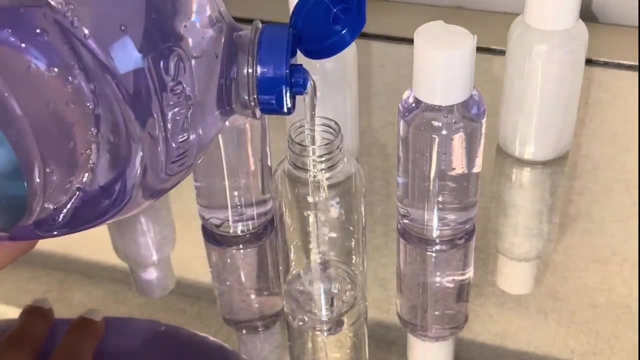 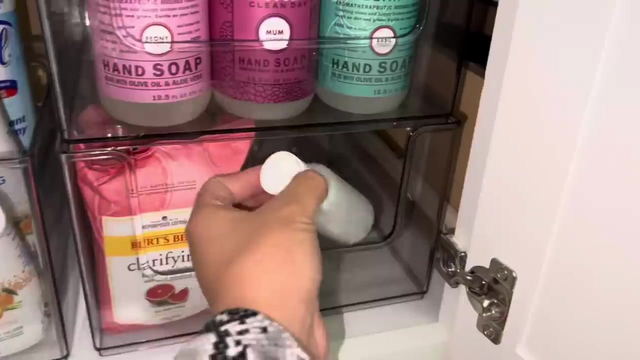 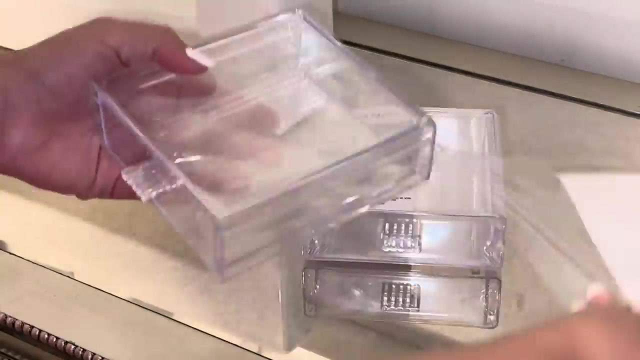 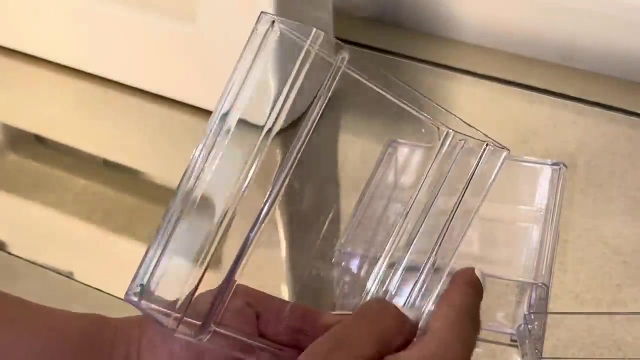 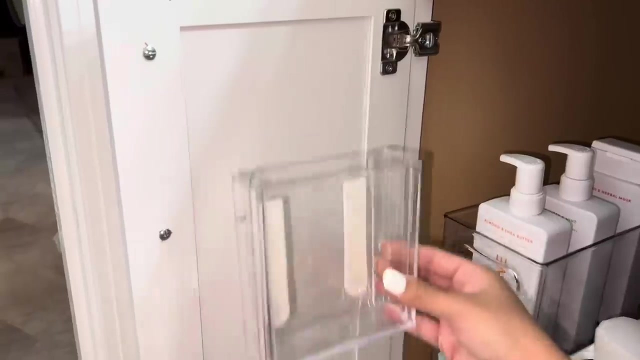 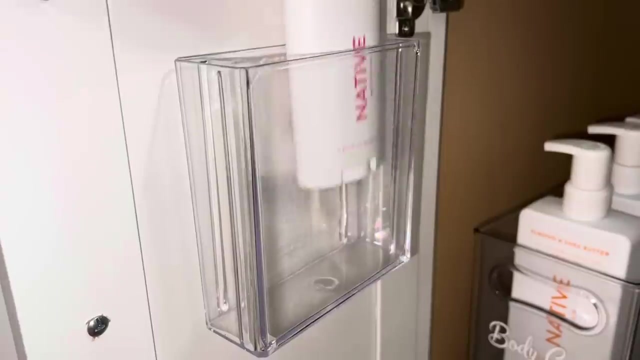 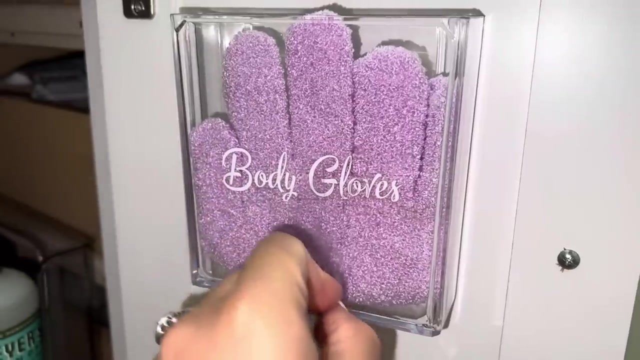 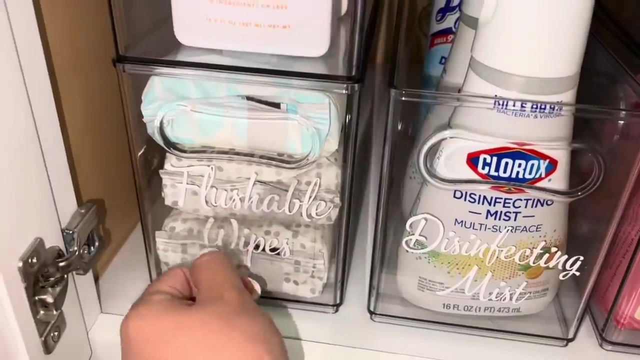 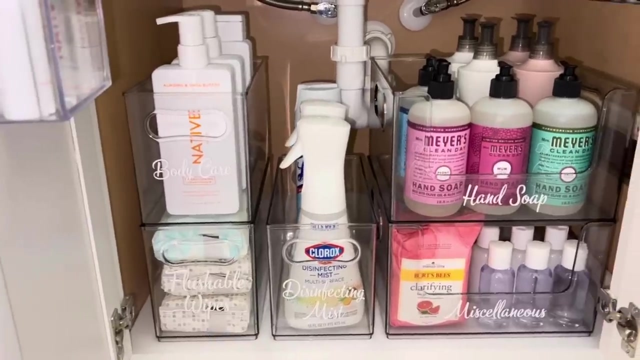 I decided to make this a little smaller and favored the entire room with a little bit of space. Thank you, Thank you, Thank you. Here's how the guest bathroom cabinet turned out. It's such a huge difference and I'm so happy that my guests can now access. 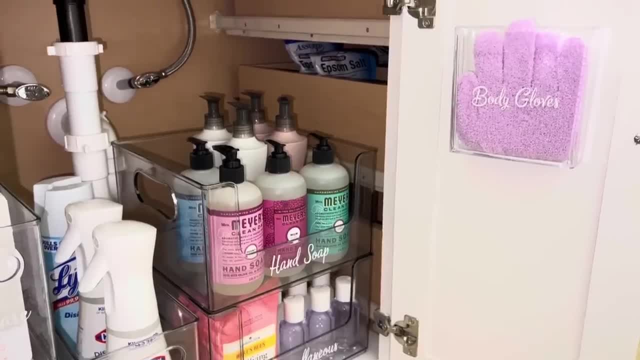 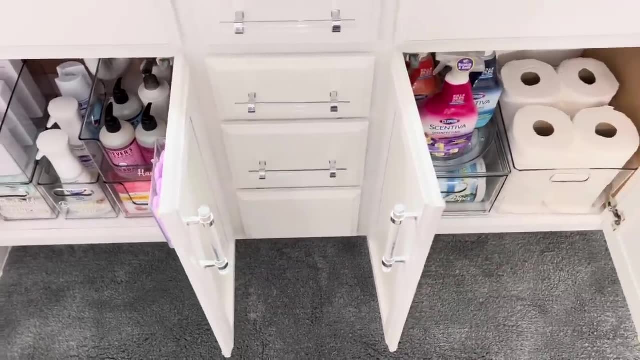 and see anything they need. This organization day was a huge success and I would love to hear what y'all think in the comments of this bathroom transformation. I would also love to hear what videos you want to see next, so I can start planning those for you guys. 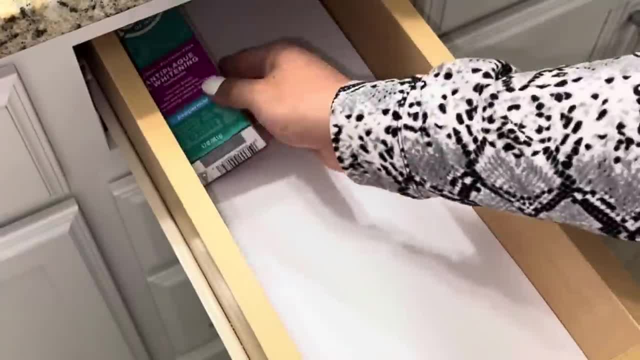 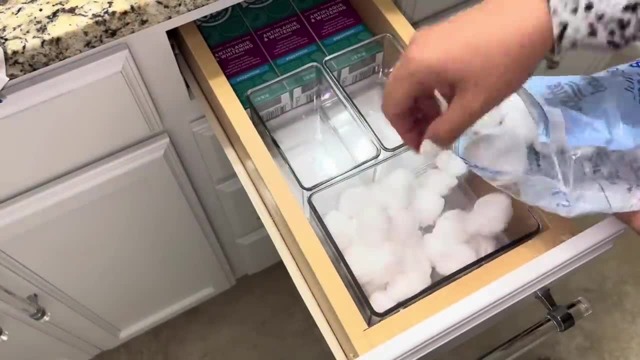 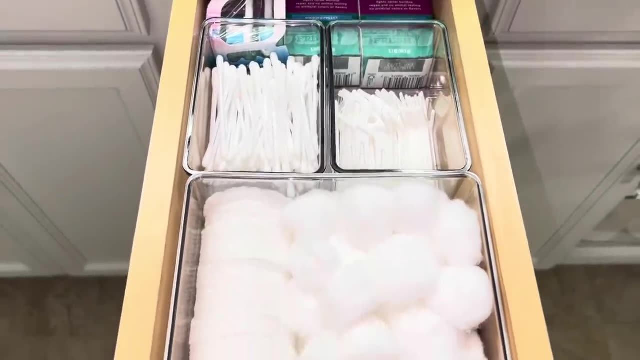 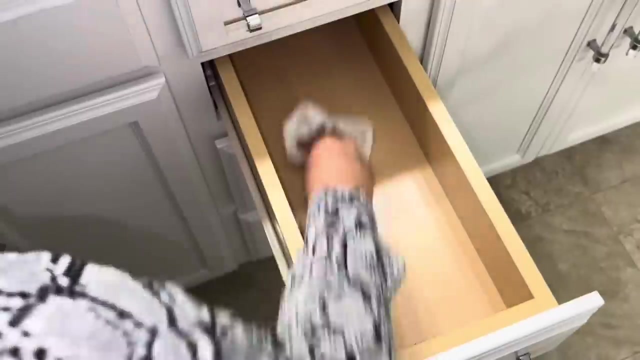 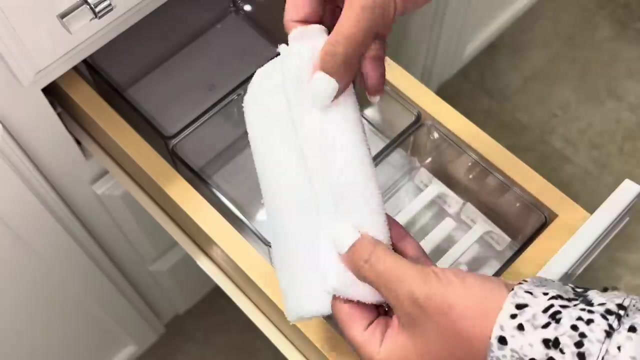 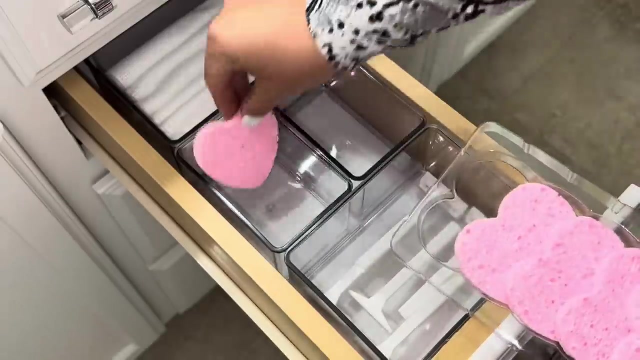 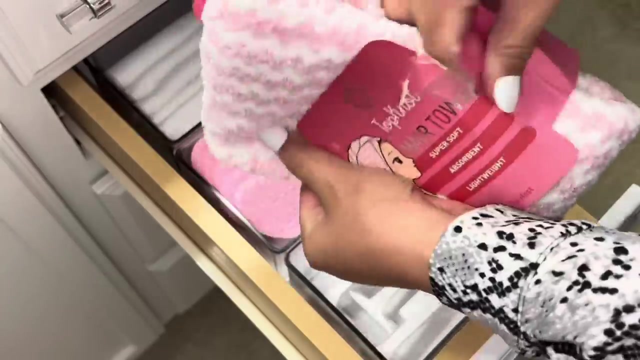 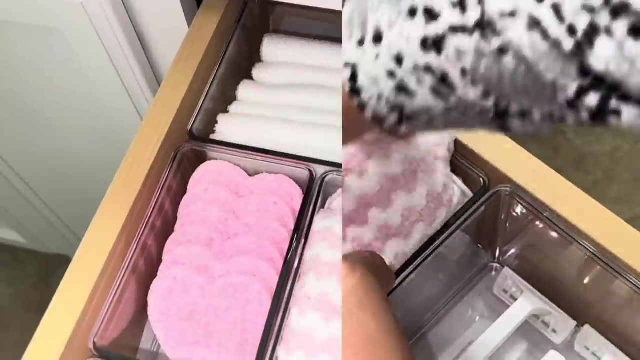 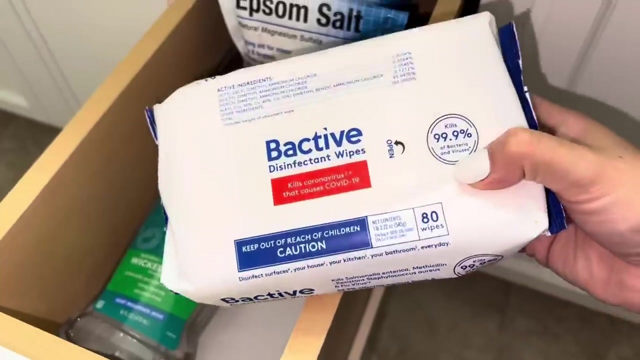 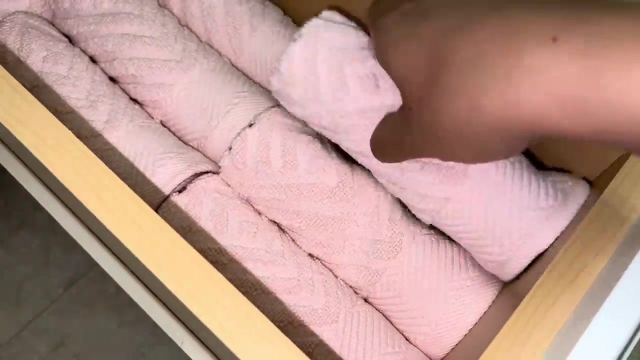 Thank you, Thank you. Remember to go check out Ritual and see the amazing vitamins they offer for you and your loved ones. Use my code LGQUEEN20 to receive 20% off your first month. The direct link is in my description box.